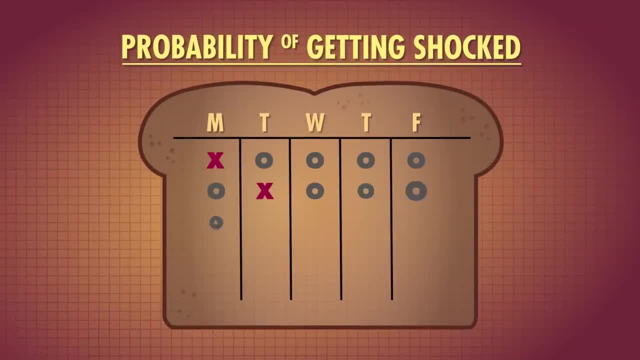 days of the week. If we represent a shock with an X and a non-shock day with an O, the possibilities for your week look something like this. So let's look at the probability of getting one shock and four non-shocks using the multiplication. 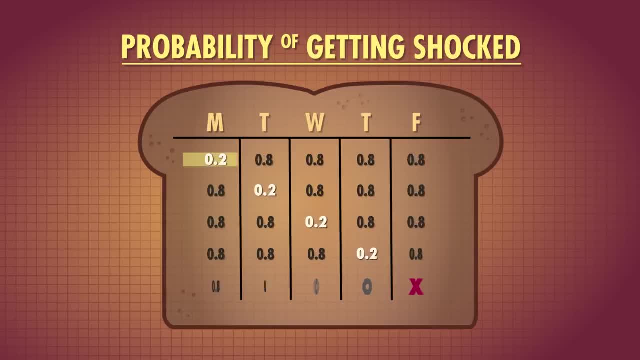 rule. Let's look at the probability of only getting shocked. on Monday, The probability of getting shocked is 20%, so the probability of not getting shocked on Tuesday is 80%, And similarly, on Wednesday through Friday, there's an 80% chance each day of not getting shocked. 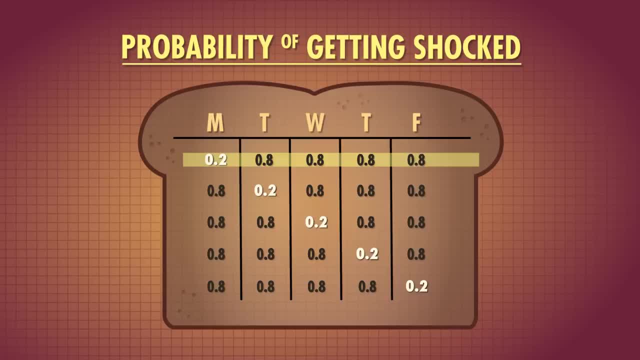 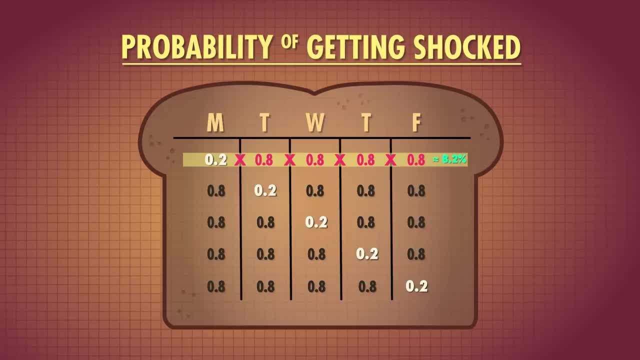 of the week. So now we've got to calculate the rest of the one-shock options. The probability of getting shocked only on Tuesday is the same, about 8.2%. since order doesn't matter in multiplication The probability of the Monday-only option or the Tuesday-only. 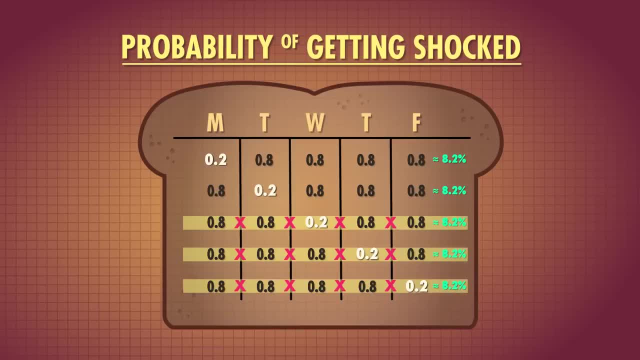 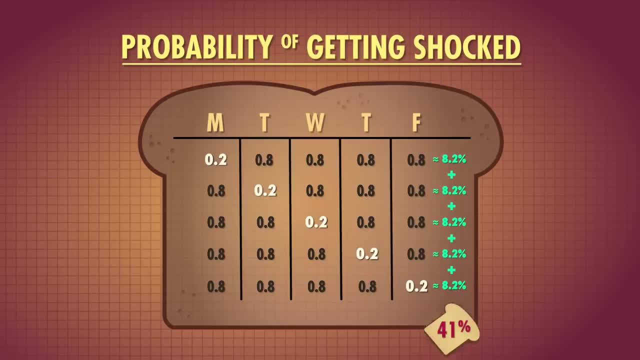 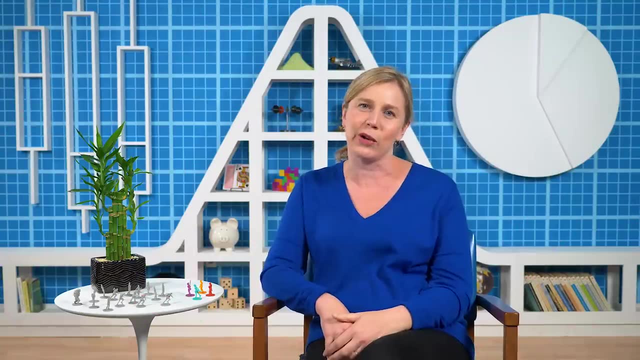 the 8.2% chance of just one shock. That's a 41% chance of getting shocked ONLY once this work week. so you decide to risk it. That was a lot of work just to figure out whether it's a good idea to have toast. 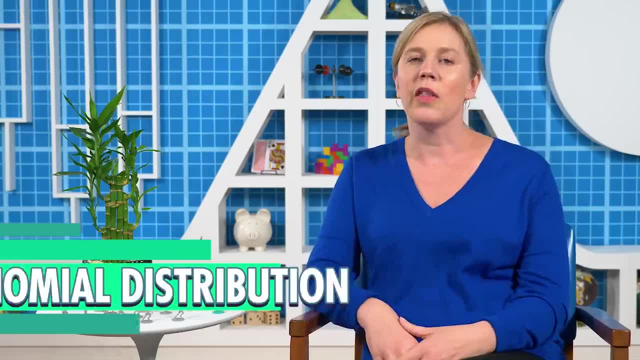 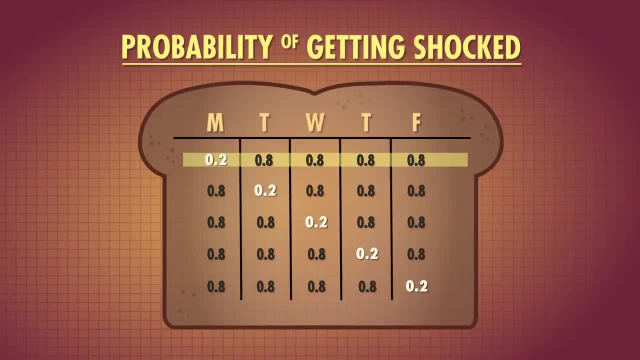 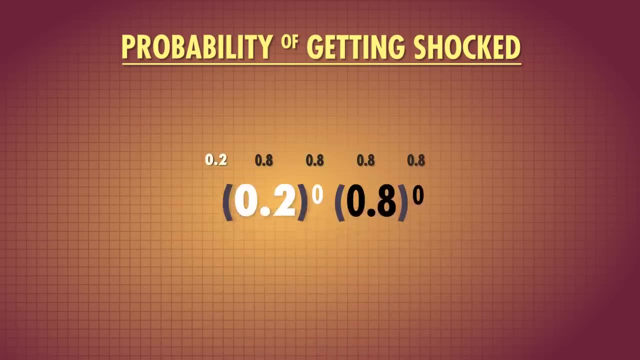 Thankfully there's a more compact formula. The formula called the binomial distribution formula takes the math we just did and simplifies it. In our toast example, we first figured out the probability of only getting shocked once. To do this, we multiplied each day's probability together. Let's use exponents to make this. 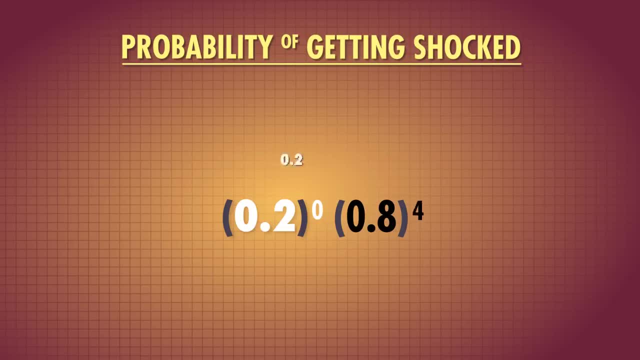 formula a little bit shorter. We can combine all the .2's and all the .8's to give us this: That's about 8%. Notice that the two exponents add up to 5, the total number of days. This formula works. 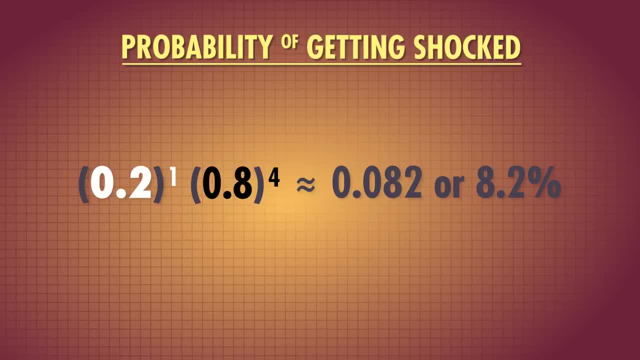 for finding out the chance of getting shocked only once, but we can also use it to find the chance of getting shocked another number of times. For example, the probability of getting shocked ONLY on Tuesday and Wednesday would be this: .02, or 2%. 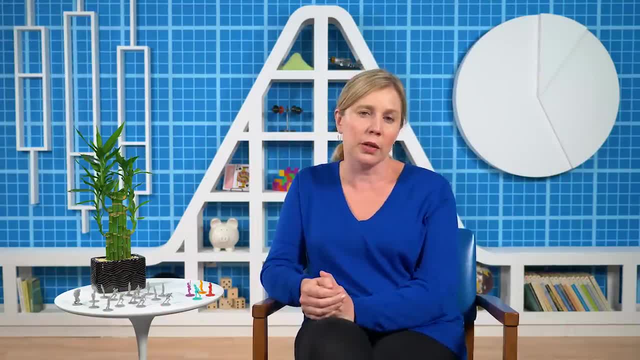 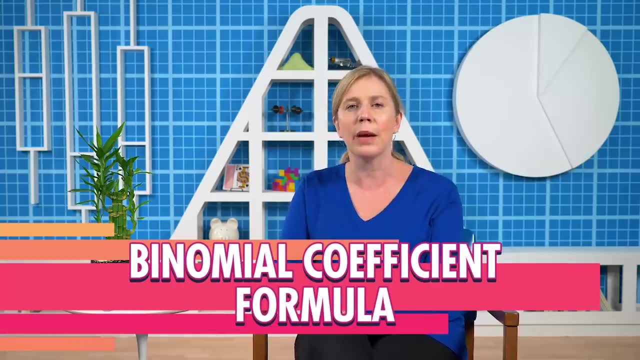 We also need to account for the number of ways that getting shocked once or twice in a week can happen. To do this, we'll use a very useful formula, the binomial coefficient formula, from a field of math called combinatorics. The binomial coefficient formula makes it. 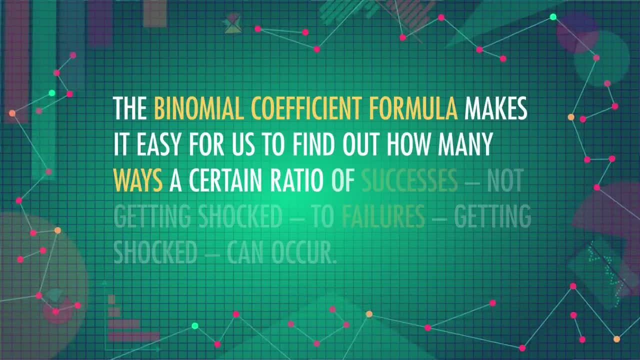 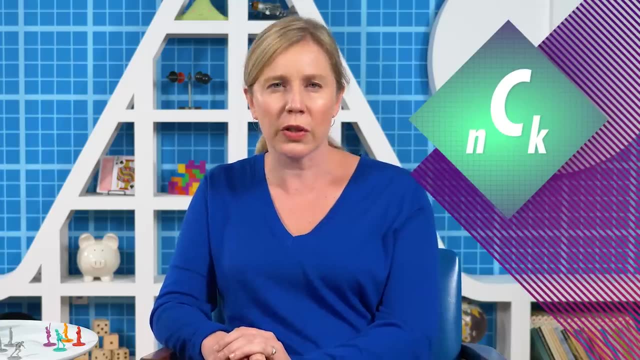 easy for us to find out how many ways a certain ratio of successes- in this case not getting shocked- to failures getting shocked- can occur In general form. it looks like this in choose k, But you also read it as we have in things: 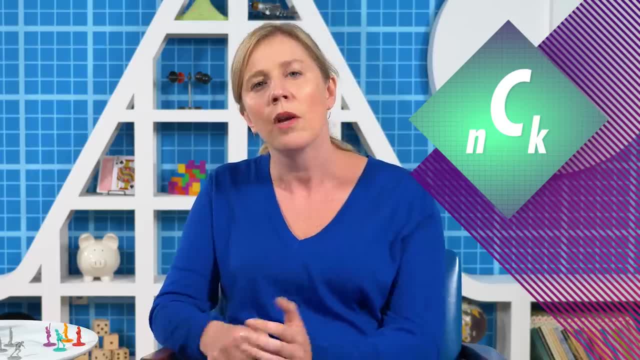 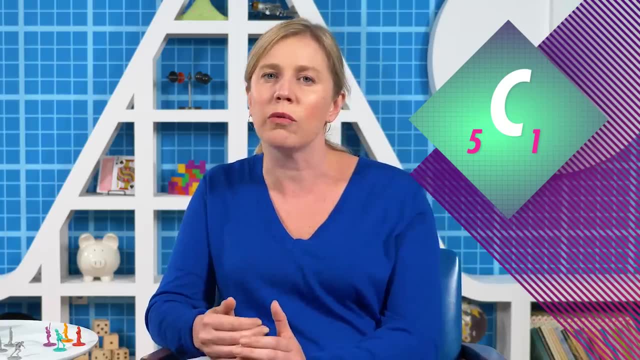 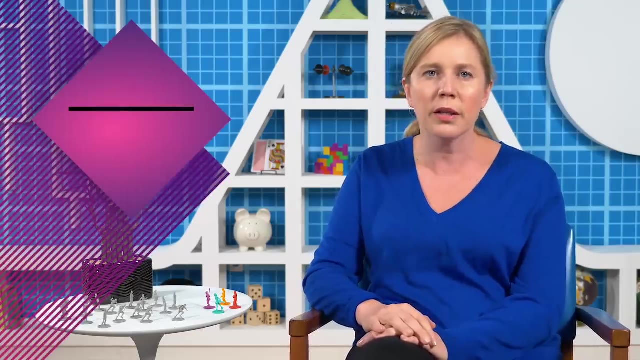 count the number of different ways. we can choose k of them For our toast. example. 5 choose 1 is 5.. That is, there are 5 different ways. we can only receive one shock from our toaster this week. The math behind this snazzy formula uses a lot of factorials which are the product of 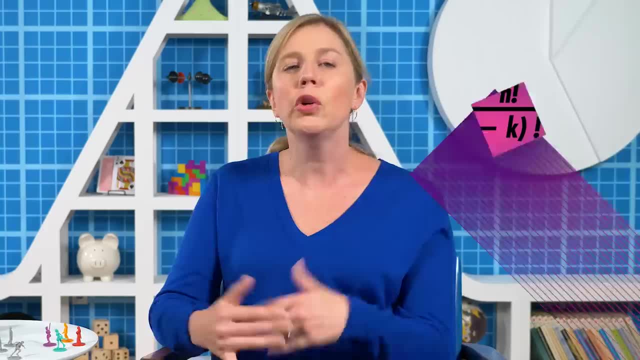 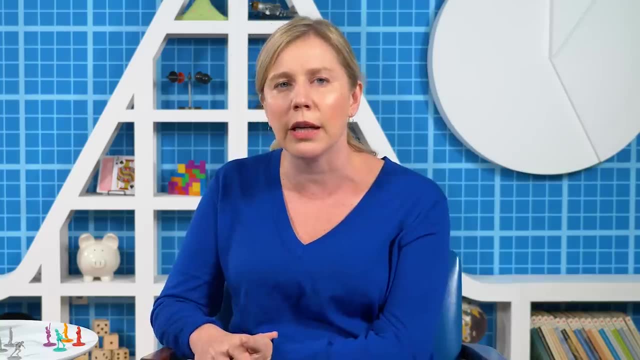 an integer and all the integers less than it. It looks like this: You remember factorials? because they're the ones that look like they're always shouting: See the exclamation marks. We won't dig into this formula here, but for more information. 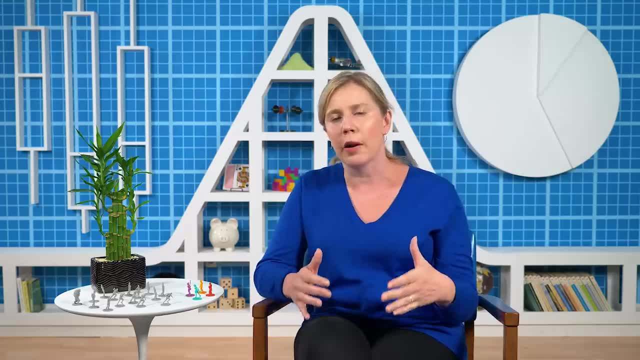 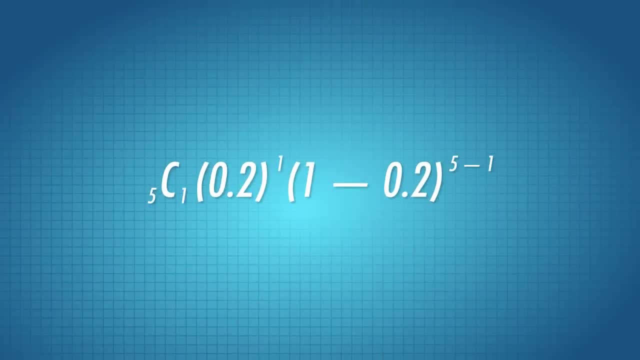 we'll link some resources in the description. Now we have all the pieces of our binomial distribution formula. Let's put them together: First the binomial coefficient, which tells us how many ways we can have one shock and four non-shocks, And then our shorthand multiplication of probabilities. We put it together and we 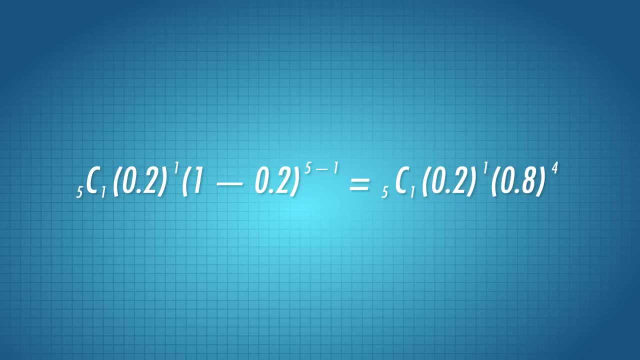 have a full-blown formula for calculating the probability of getting shocked. This is the probability of getting shocked on 1 out of 5 days this week, about 40%. It took us a while to get here, but now we have a general formula for calculating any. 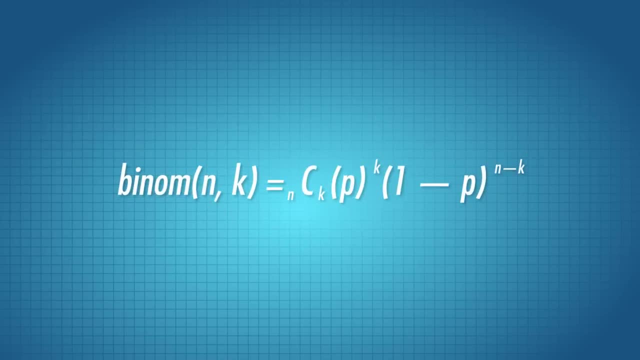 similar probability. If p is the probability of our event happening, then here's our formula. For example, supposing there's an equal chance of having a boy or a girl, If we want to find out the probability of a couple having 3 girls out of 5 children, we can simply plug: 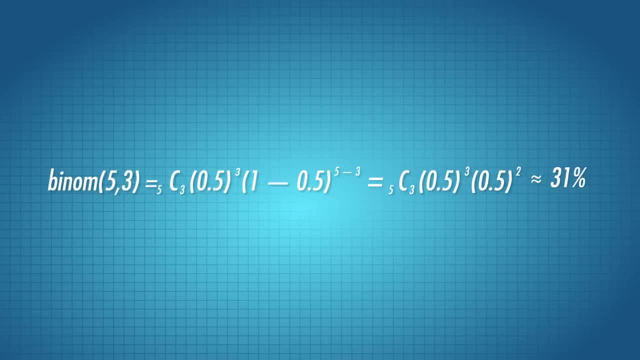 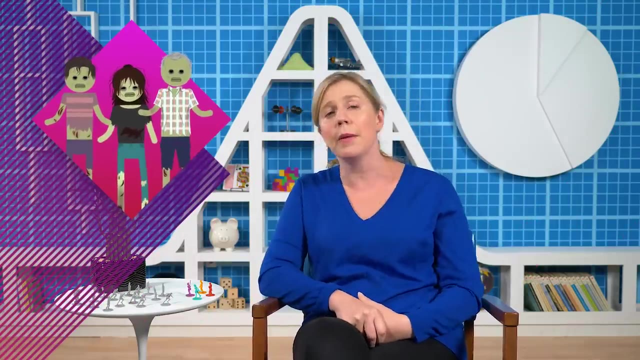 our numbers into the equation. We do that and we see there's about a 31% chance of 3 of their 5 children being girls. And now we get to the zombies. It's the beginning of the zombie apocalypse, and you 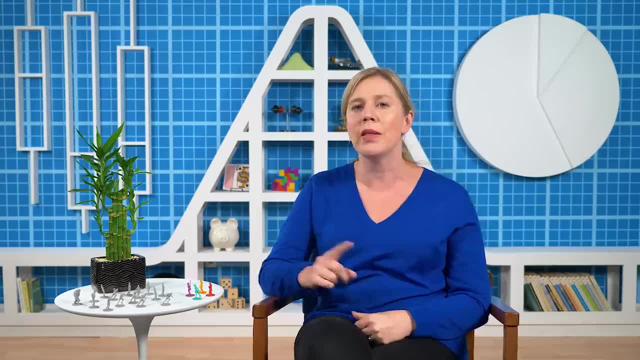 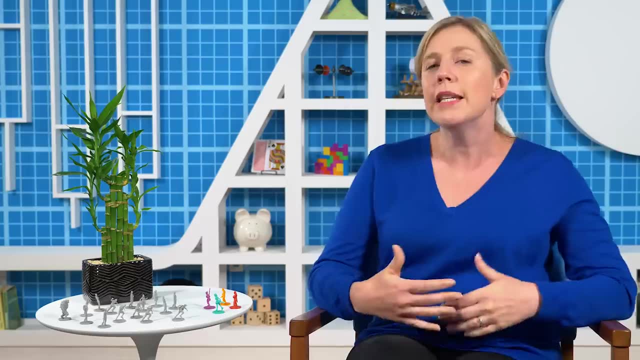 thankfully still have your brains, But there's a bunch of people between you and the nearest shelter and you want to know how likely it is that none of them have been bitten and infected with the zombie virus. Since you can't always tell if a person is infected right away, you decide to use 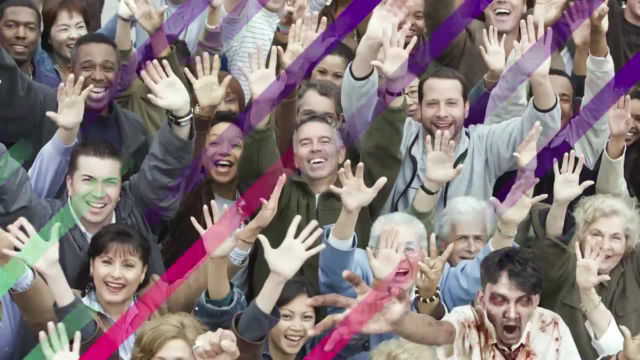 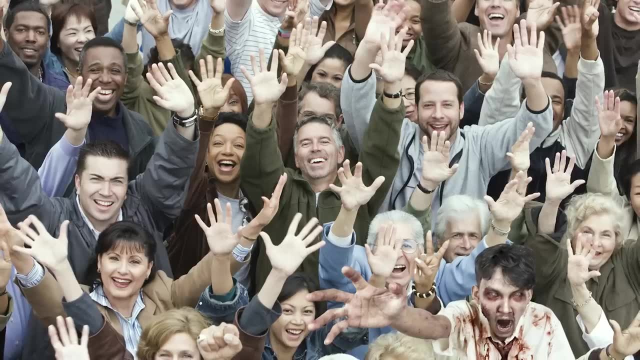 your binomial probabilities to calculate your chances. It's early stages, so right now there's only about a 5% infection rate in the population. That means the probability of someone being a zombie is about 5% and the probability of not being infected is still about 95%. 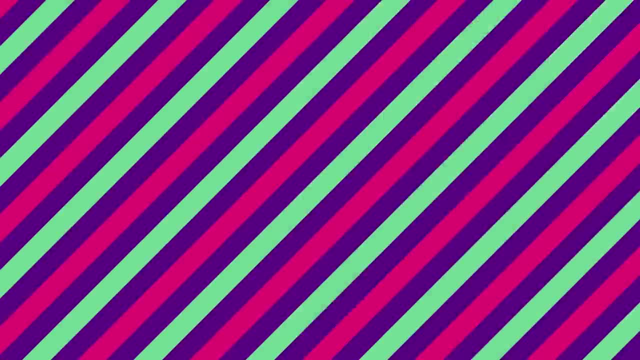 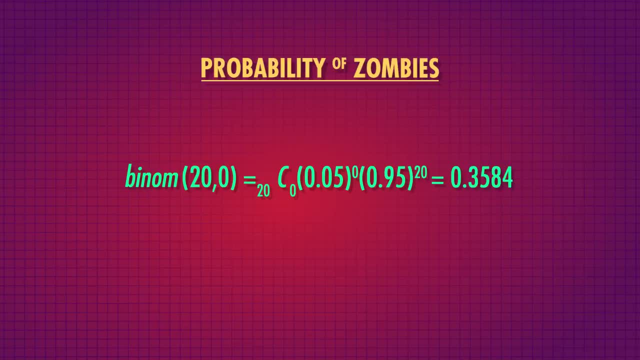 Peeking out at the crowd that stands between you and the shelter, you count 20 people. Plugging these numbers into our formula, we can see that there's about a 36% chance none of the people you'd encountered on your run to safety will try to eat your brains. 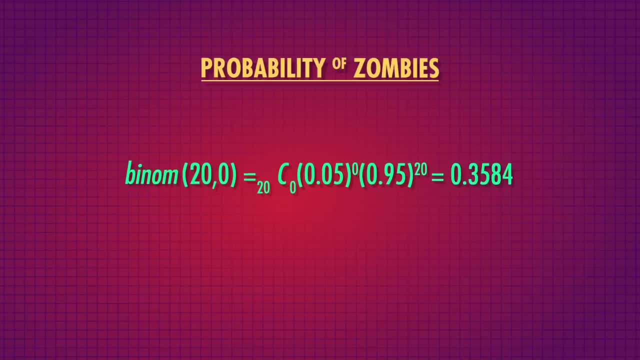 Those are pretty good odds. and you're fast, You know you could probably safely reach the shelter even if there were one or two zombies. So let's calculate the probability of a zombie being infected by a zombie. Let's calculate those probabilities as well. 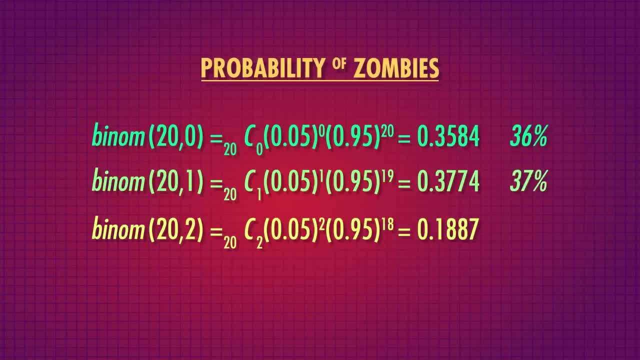 There's about a 36% chance of meeting no zombies, about a 37% chance of having only one easily dodgeable zombie and about an 18% chance of having to outmaneuver only two. That means that cumulatively that's about a 91% chance that you'll be able to sprint. 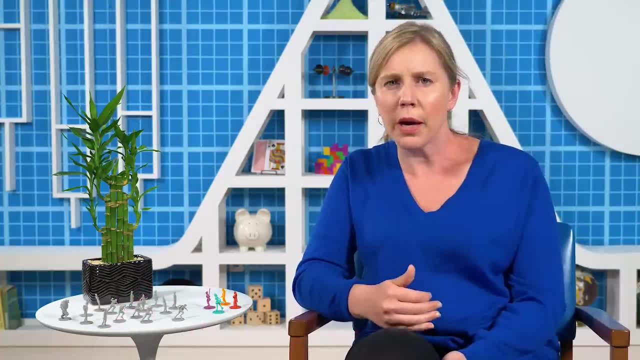 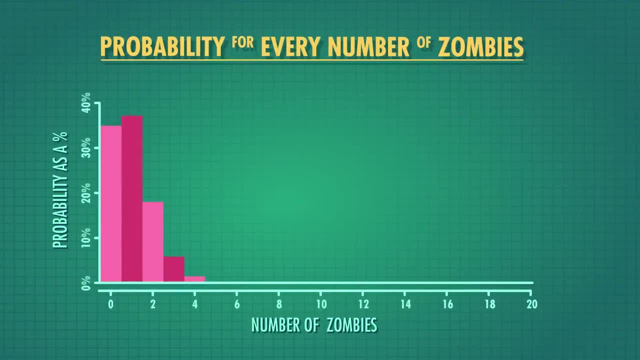 your way to safety. We could calculate the probability for every possible number of zombies from 0 to 20.. If we did, we would get the discrete distribution for this specific type of probability. So the probability of a zombie being infected by a zombie is 5% of the probability of a 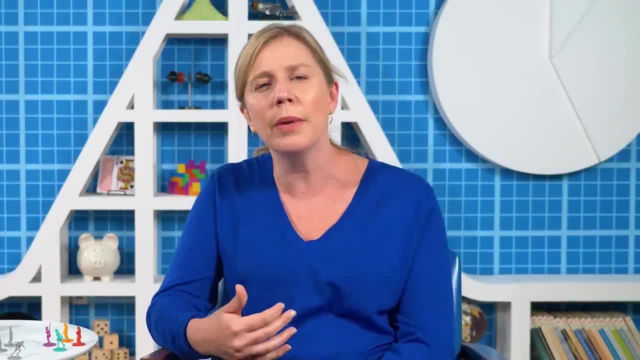 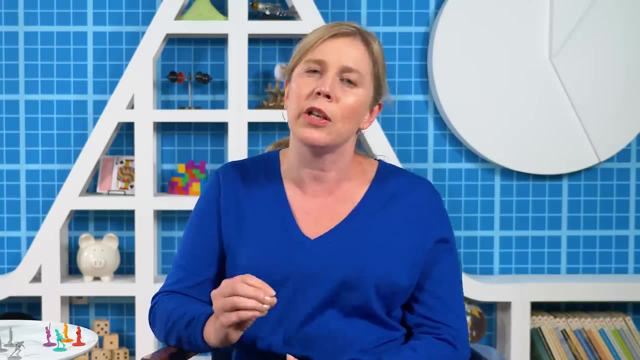 zombie being infected by a zombie. But in a more general sense, I also want to know how many zombies I would expect to confront on average, just so I can prepare. I could try to guess the mean by looking at the graph of the binomial distribution for all the possible cases. 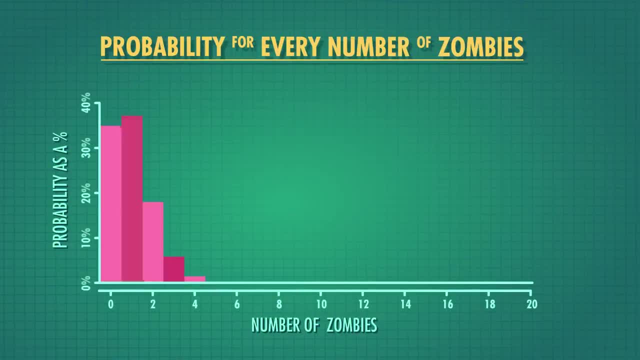 Just by eyeballing it I'd say the mean of this distribution is around one And it is The actual formula to find the mean of a binomial distribution is in the number of events we're looking at times p, the probability of what we're interested in, the probability. 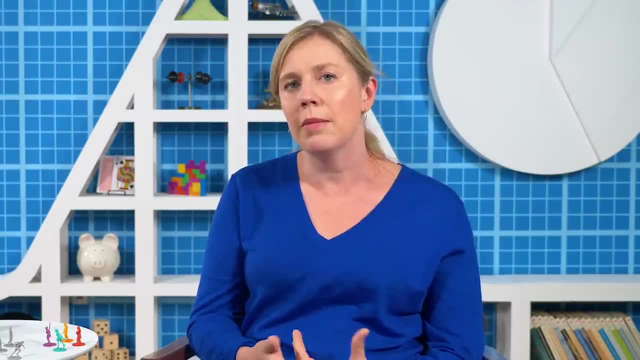 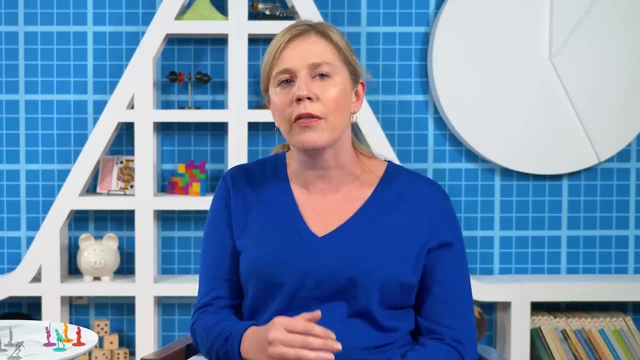 of being a zombie. Since the probability of being a zombie is 5%, it makes sense that, on average, about 5% of any population will be zombies. Since we have a group of 20,, we expect about 5% of 20, or one zombie infection on average. 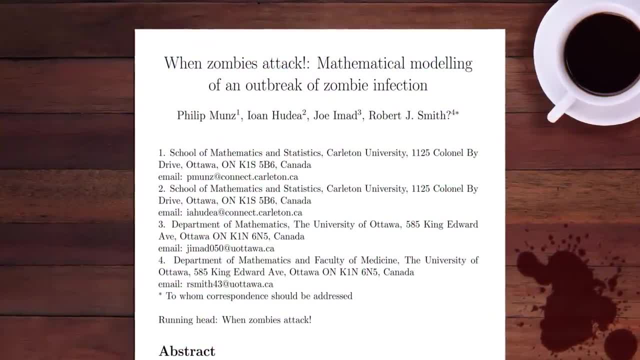 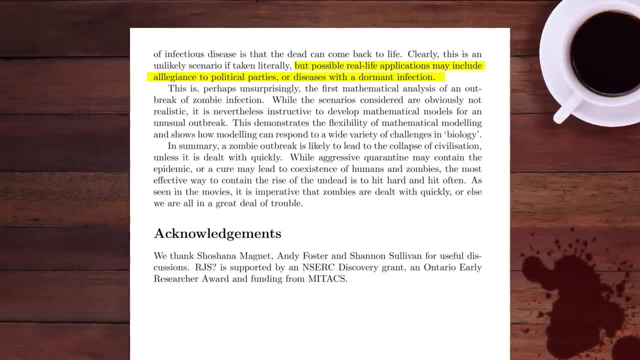 While zombies are probably not on your day-to-day list of concerns, this kind of calculation might be Important. public health issues such as the spread of pandemics, lockdowns and a pandemic level of viruses can be modeled using a similar approach. 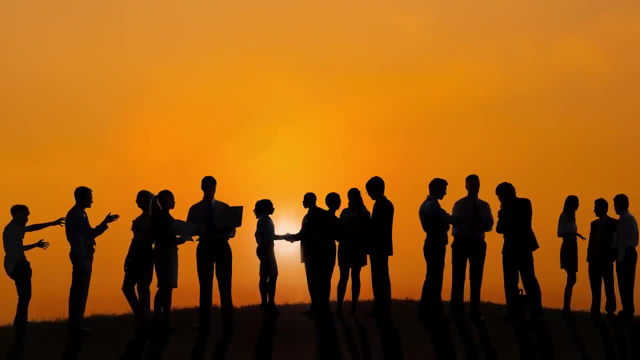 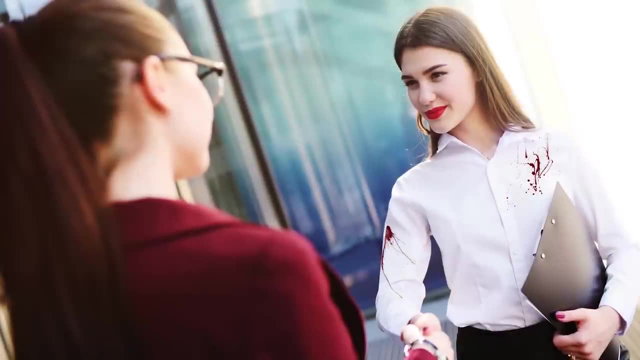 We could just as easily calculate the probability that of the 40 people you shook hands with at the zombie apocalypse meetup, two or fewer had the cold that's been going around. Or we could calculate the mean number of cold-infected people you could expect to shake hands with. 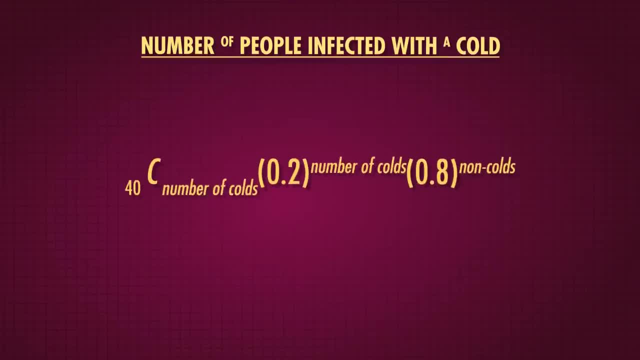 at any given meeting. If the probability of having a cold at that given moment in the population is 20%. the probability of only two or fewer people having a cold is only 20%. If the probability of having a cold at that given moment in the population is 20%. the 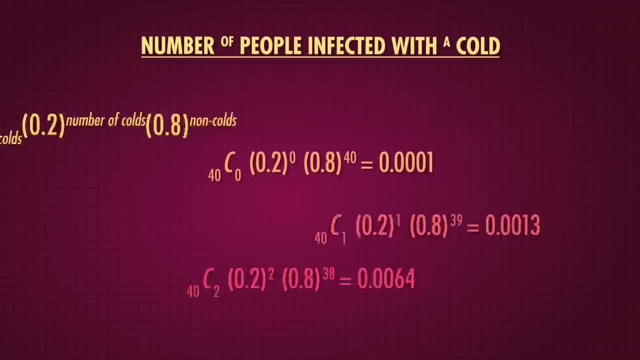 probability of only two or fewer people having a cold is only 20%. If the probability of having a cold at that given moment in the population is only 20%, the probability of only two or fewer people having a cold is only about 0.7%. 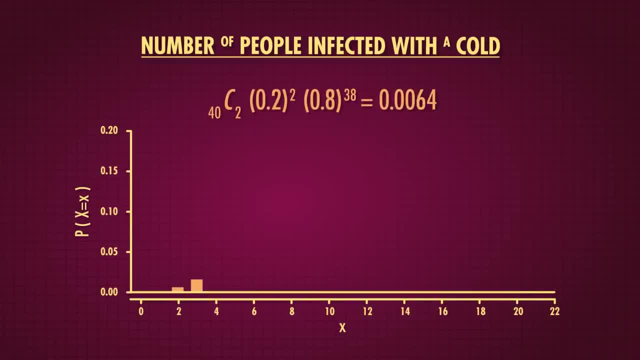 From the binomial distribution, with 40 people and a 20% chance of having a cold, we can see that it's much more likely that more than two people will have the sniffles. In fact, you'd expect 20% of 40, or 8 people to have a cold at any similar meeting with. 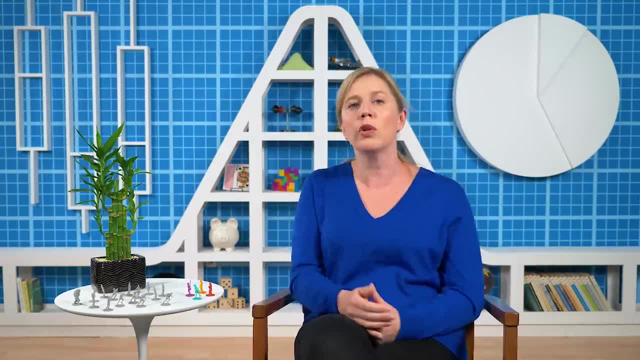 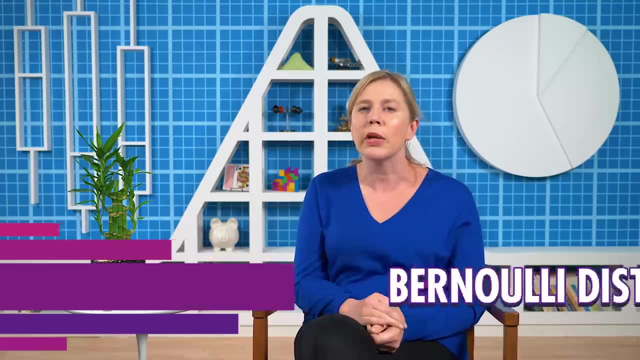 40 people. A special case of the binomial distribution with only one trial or just one event, a single coin flip, for example, is called the Bernoulli distribution. It represents the probability of getting either a 60% chance of having a cold or a 50% chance. 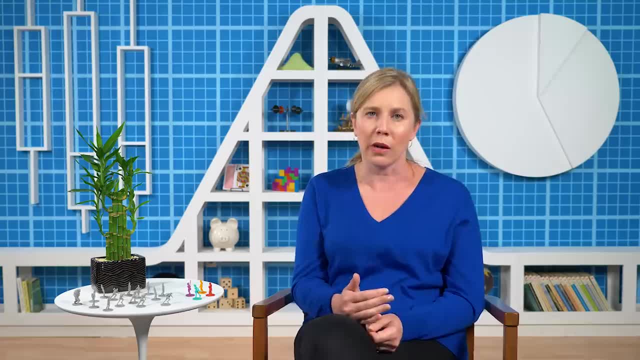 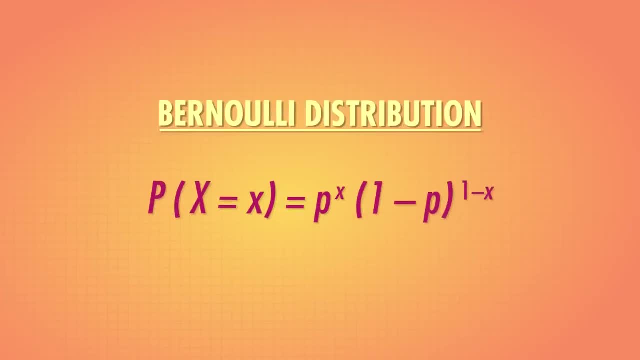 of having a cold. If we have a success or a failure, our outcome x can either be a 0, failure or a 1, success. The general formula for the Bernoulli distribution, where p is the probability of success, is: 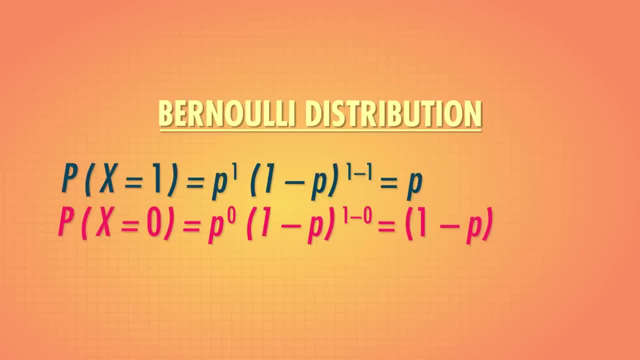 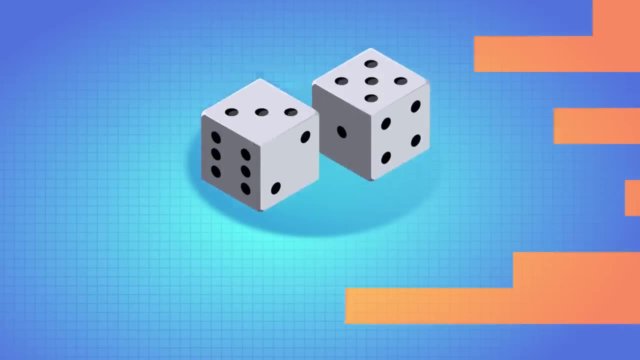 this And by plugging in 1 or 0, we can see, the probability that our outcome is a success is p and the probability of a failure is 1 minus p. For example, if the probability of rolling an odd prime number- a, 3 or a 5, on a single 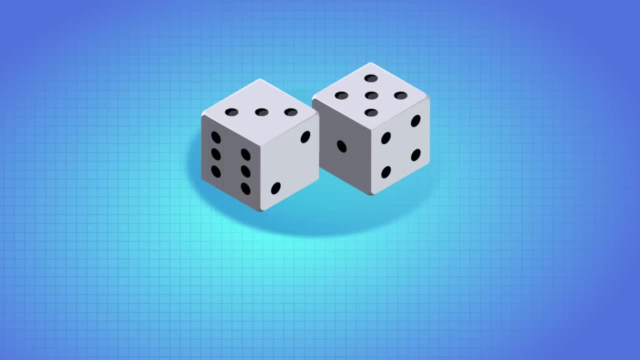 dice roll is about 33.33%. That's the probability. Then the Bernoulli distribution for rolling a prime number would be the probability of rolling an odd prime to the x power multiplied by the probability of not rolling an odd prime to the 1 minus x power. 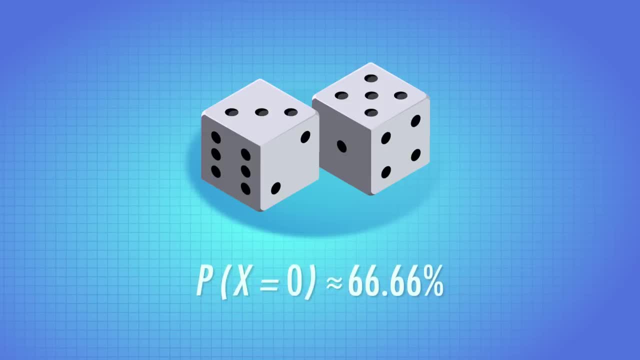 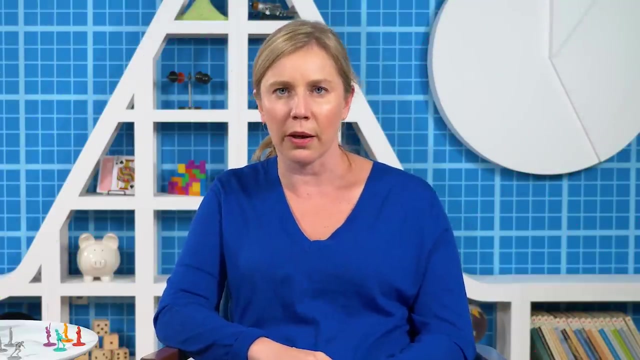 When x is 0, a failure, then the probability is 1 minus a third, or around 66.66%, And when x is 1, a success, the probability is around 33.33%. Though relatively simple, The Bernoulli formula is a useful building block. 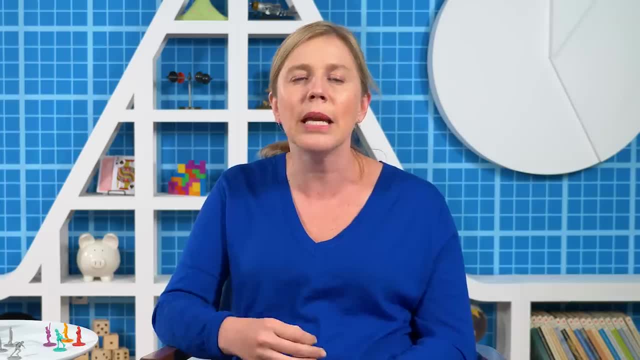 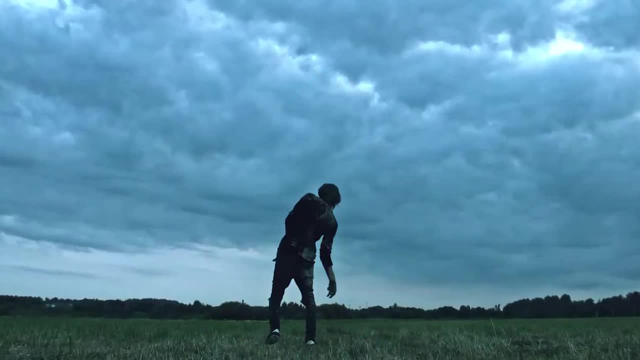 For instance, you can think of the binomial probabilities that we did as many Bernoulli trials, one after another, And in reality that's what they are. Alright, let's get back to the zombies. Things have gotten much, much worse. 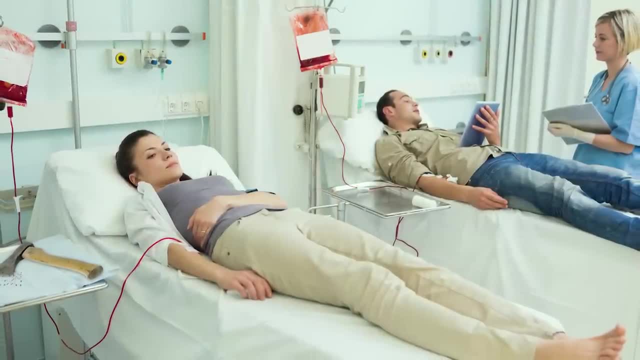 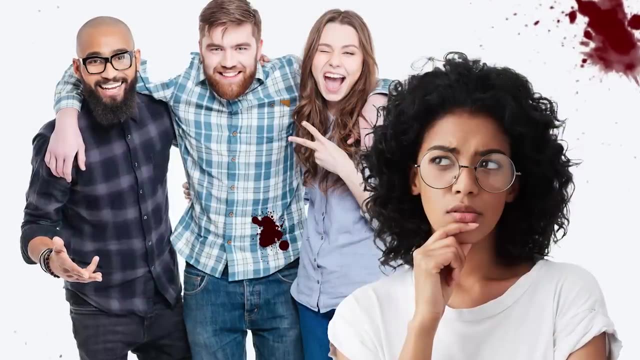 Zombies are everywhere. You're injured really badly, You need a blood infusion, And you need so much blood that you'll need some from all three people around you. Luckily, you're type AB positive, so you can get blood from any blood type. 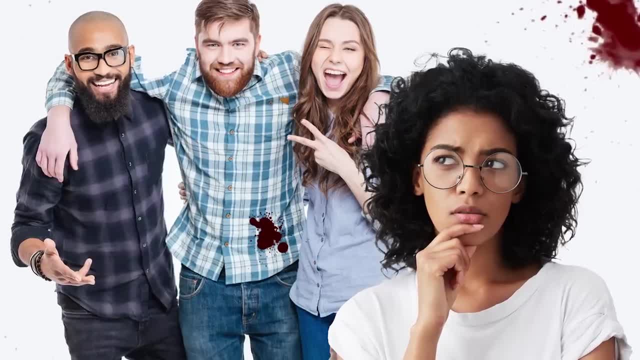 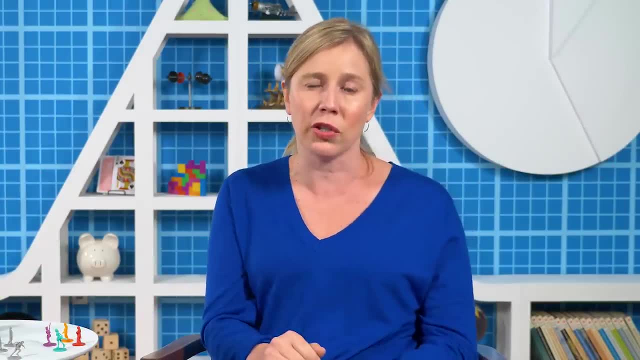 But you have something wrong And you have something else to worry about: The latent zombie virus. All three of your buddies seem okay, but you heard on the radio the population now has a 30% infection rate, so there's a 30% chance they're infected with the zombie virus and are just asymptomatic. Luckily, the human immune system can handle the virus in very small doses, so you'll be okay if at least two thirds of the blood is clean. What are the chances you're going to survive the infusion If someone has a latent zombie infection? 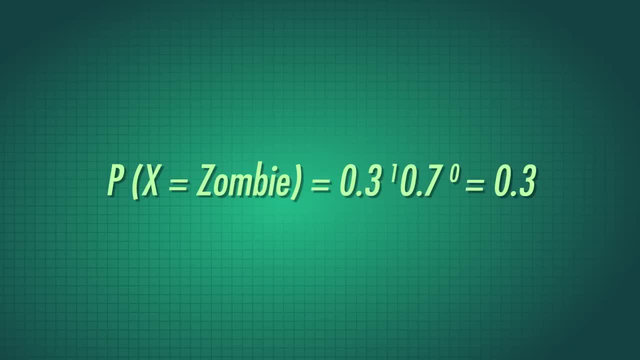 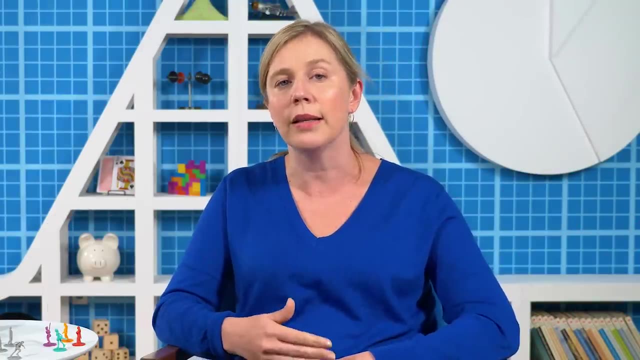 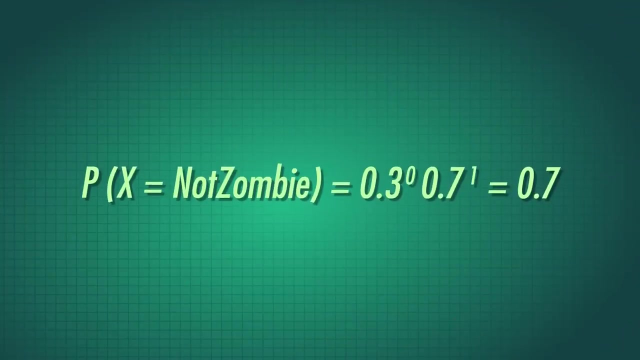 then the Bernoulli trial would have one success and zero failures. giving this formula for the trial, Which, as we expect, means there's a 30% chance that one random person has a latent zombie infection And every person who is not infected is considered to be one failure and zero successes, which 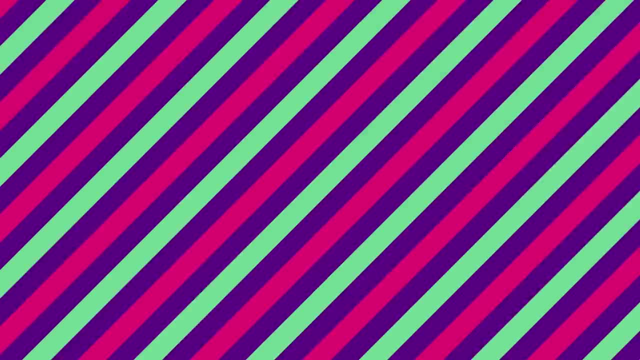 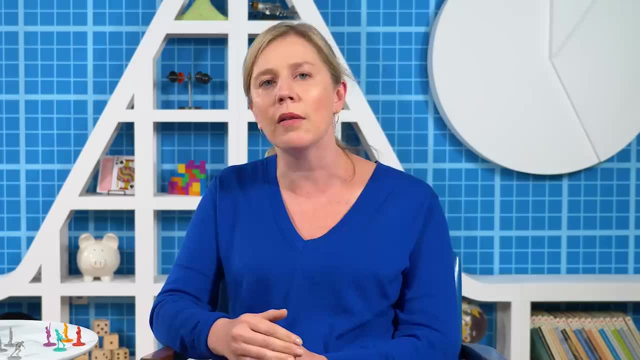 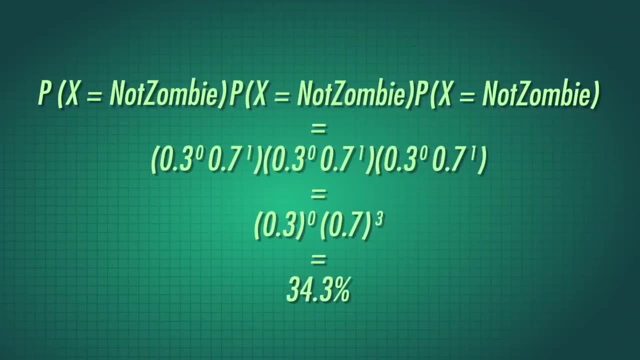 has a 70% chance based on this Bernoulli formula. We can use different combinations of these two Bernoulli formulas and multiplication to figure out the probability that you'll remain uninfected after your much-needed blood transfusion. You'll be fine if no one has any latent zombie virus and we can calculate the probability. 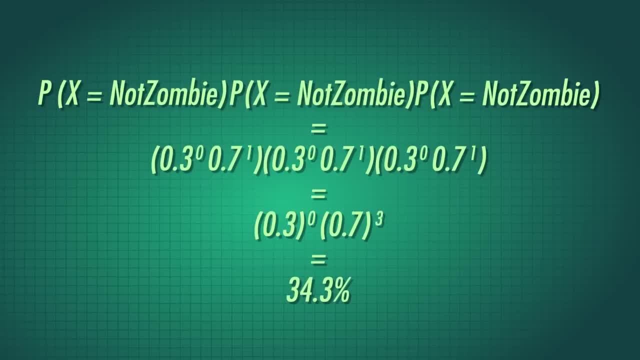 of that happening by combining three successful Bernoulli trials And this looks a lot like the second part of our binomial formula because it is A 34.3% chance of survival is kinda low, but don't forget, you'll also be okay, if only.